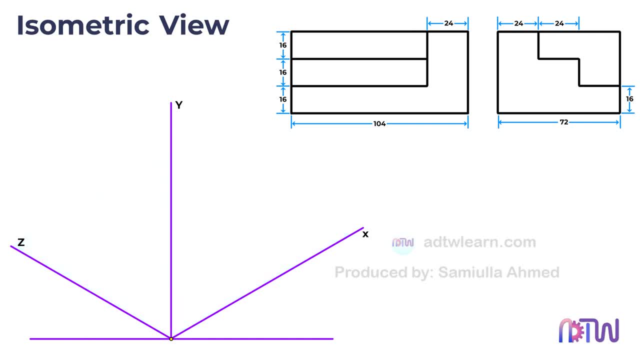 so that's another key point to keep in mind. On the left-hand side we see the front view of the object, while on the right-hand side we see the side view. To draw the front view, we'll use the x-y plane, and for the side view, we'll use the x-y plane. To draw the front view, we'll use the. 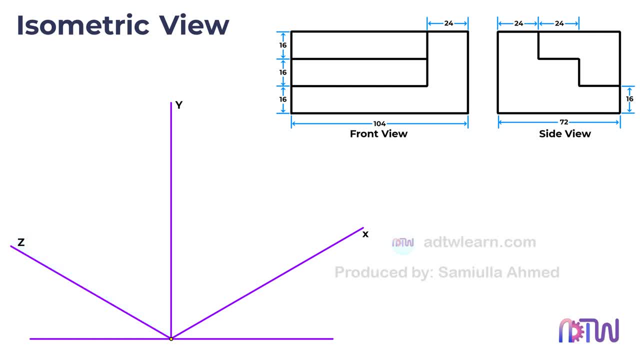 y-z plane. From the front view, we can tell that the object's total length is 104 mm and its width is 72 mm. So we'll start by drawing a 104 mm line on the x-y plane, followed by a 72 mm line on the. 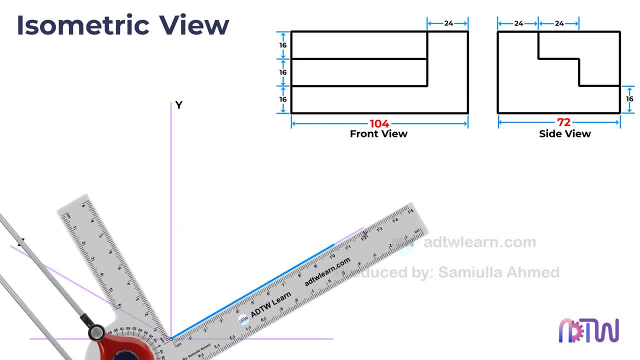 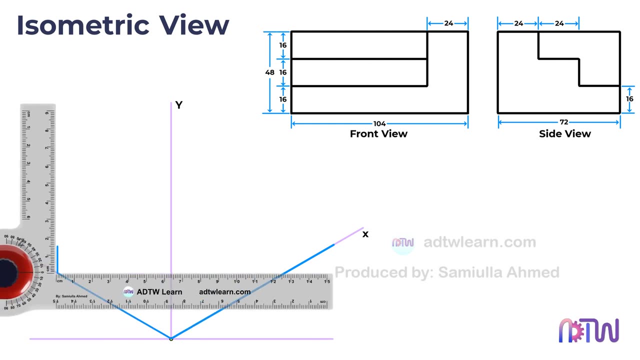 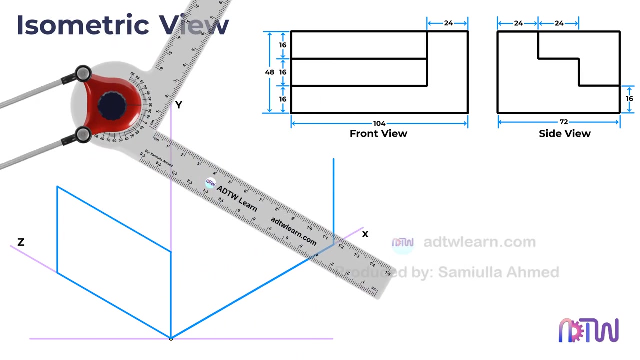 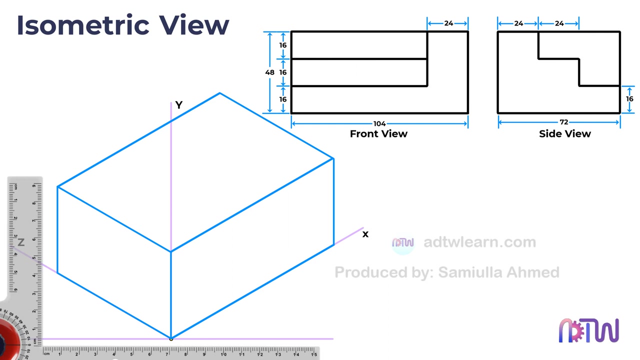 y-z plane. Moving on to the height of the object, we can see from both views that it is 48 mm. Therefore, we'll draw a line of 48 mm and construct a cuboid outline for the object. It's important to note that this cuboid is just the basic outline for the object. 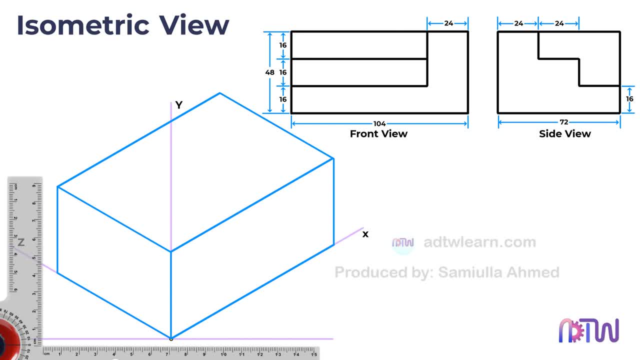 and further details will need to be added to create an accurate representation. Now that we have the basic outline of the object, it's time to add some details. We can see this part of the object. it has no solid lines. From the side view. 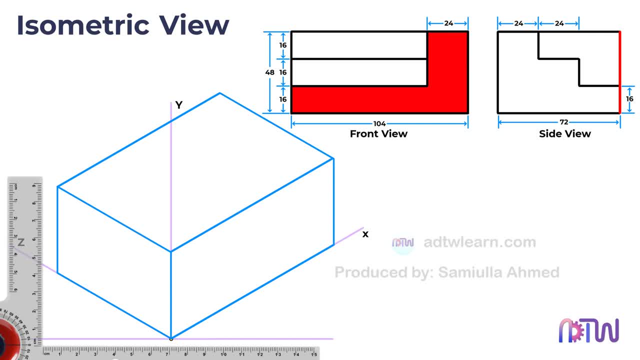 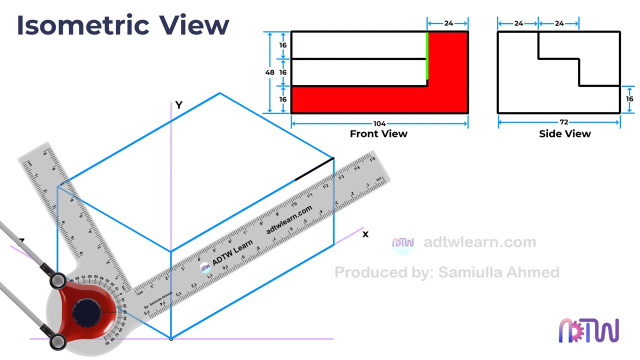 we can see that this portion is in front of the object. Hence we can construct this feature on the x-y plane. Using a drafter, draw a 24 mm line parallel to the x-y plane from this point. The length of the vertical line from this point is 32 mm, so draw a vertical line of 32 mm. 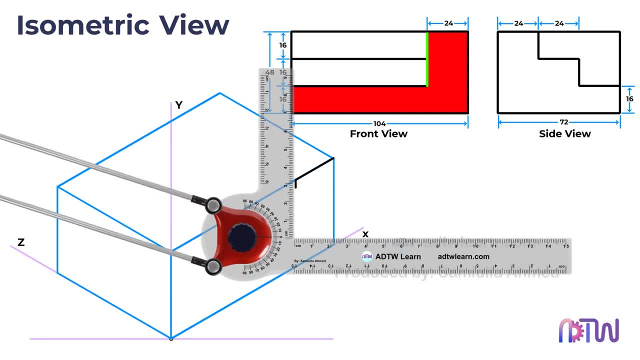 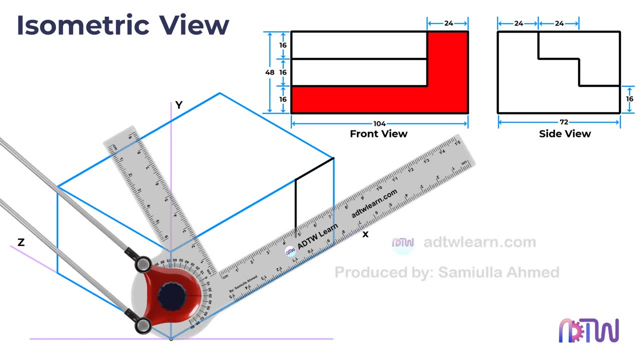 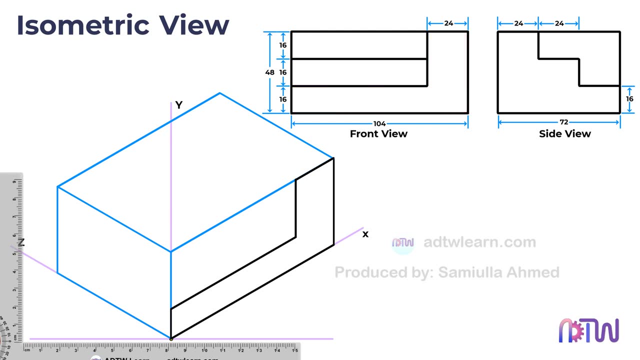 downwards from the previous line, as shown. Finally, draw another line parallel to the x-y plane up to the y-axis, as shown. This is how this feature will look in the front view. Let's proceed with adding the features visible in the side view of the object in the y-z plane. 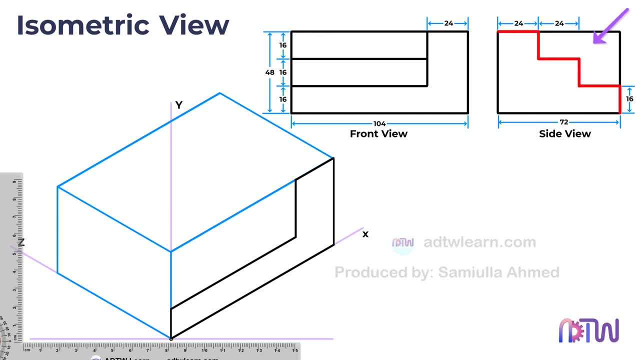 We can observe that there is a stair-like structure in the side view. To construct this, draw a line of 24 mm parallel to the z-axis. Next draw a vertical line of 6 mm. Next draw a vertical line of 16 mm, followed by another line of 24 mm parallel to the z-axis. 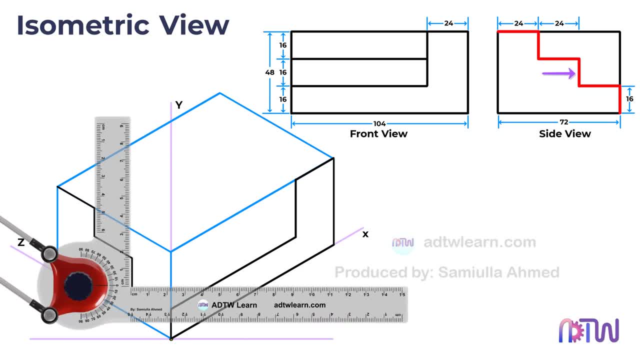 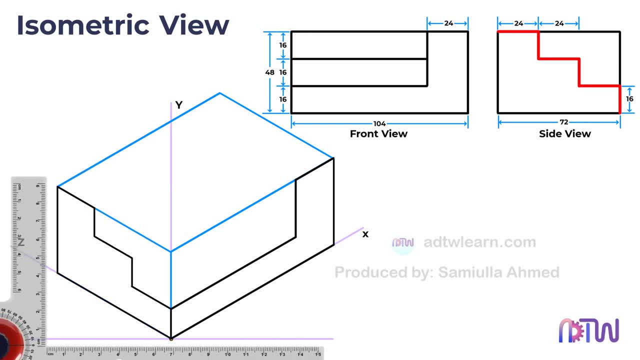 Draw another vertical line of 16 mm and finally a line of 24 mm parallel to the z-axis. This completes the side view of the object in the y-z plane. The lines in the front view represent these points in the side view, which in turn represents these: 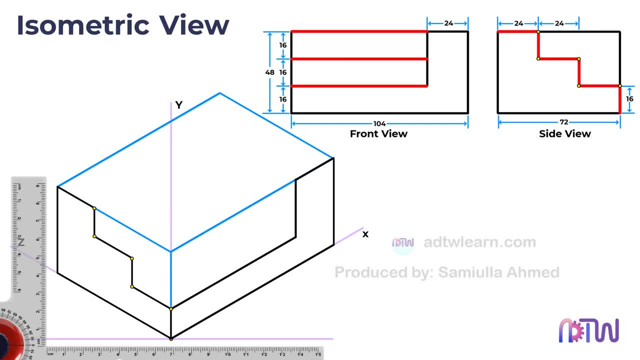 points in the isometric view. To draw these lines, we need to find their length. in the front view, The length can be found by subtracting the length of this solid structure, which is 24 mm, from the total length of the object, which is 104 mm. 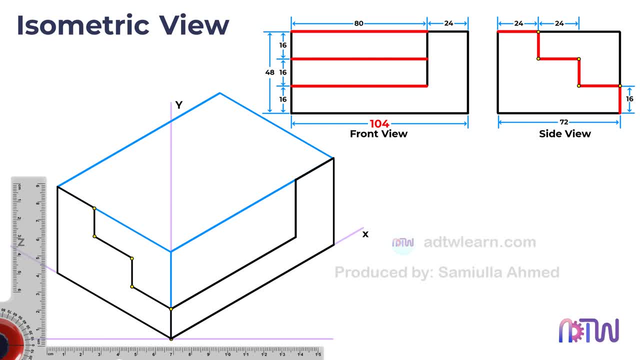 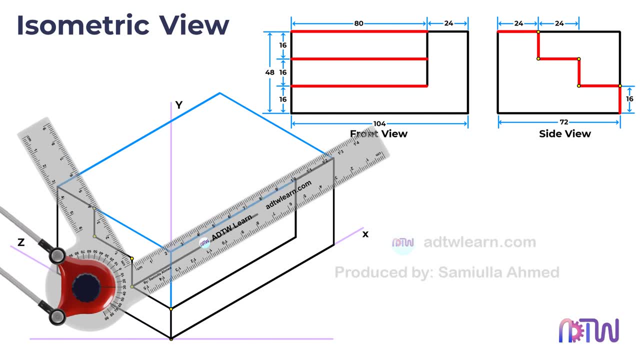 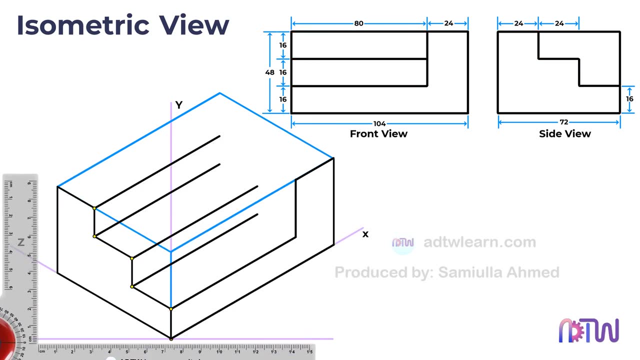 Therefore draw an 80 mm line from the points in the isometric side view parallel to the x-axis, to complete the construction of the object. After the previous step, we notice that this line in the in the side view starts from this point in the isometric view, So we can start drawing a line. 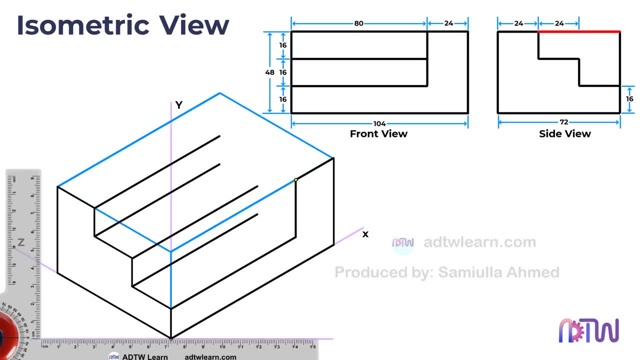 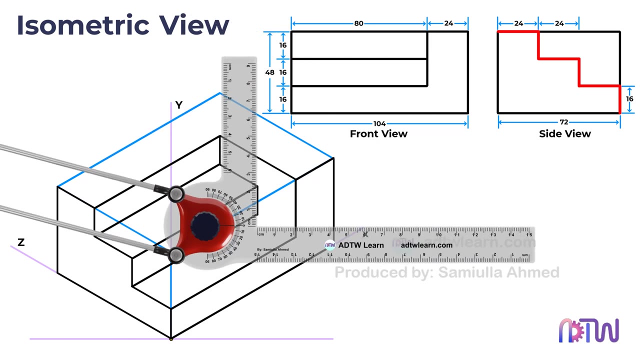 parallel to the z-axis, from this point up to the intersecting line, Moving on. the lines we see in the isometric view represent the stairs in this structure. Therefore, we will draw lines parallel to the y and z-axis to construct the stairs. This is the final isometric view of the object. 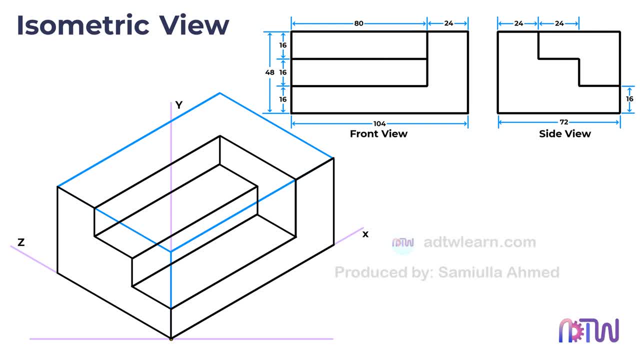 Once this is complete, we can proceed to eliminate the outlines of the structure and instead use dark lines to draw the figure. The next step in the process is to add dimensions to the isometric view. This marks the final stage in creating the isometric representation from the given. 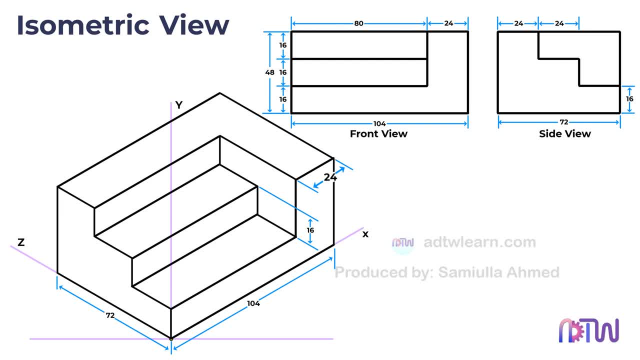 orthographic projections. I trust that this video has been instructive in demonstrating how to construct an isometric view. If you found this video helpful, please consider liking it and if you are new to my channel, ADTW Learn, please click on the subscribe. button and turn on all notifications to receive my latest videos.